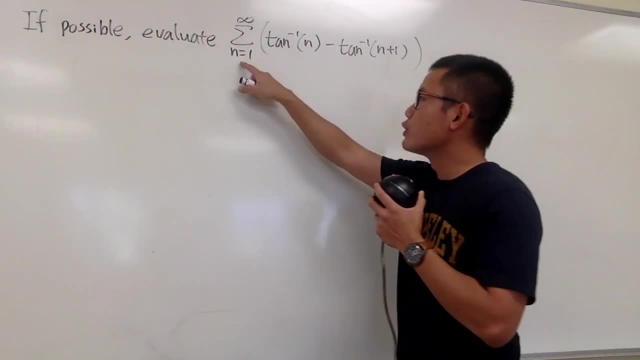 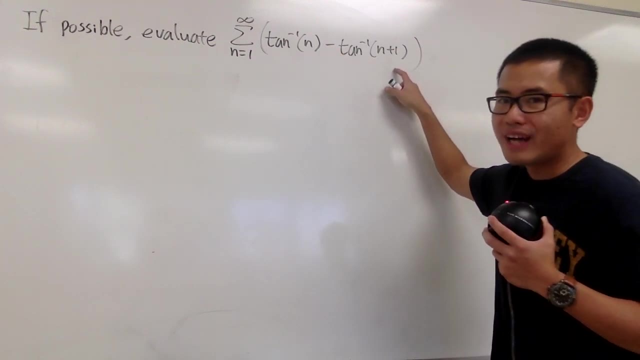 Okay, if possible, we are going to find this sum right here, the sum when n goes from 1 to infinity, and inside here we have the inverse tangent of n minus, the inverse tangent of n plus 1.. We have two things inside and this and that are the same kind, and they are just all by 1, isn't it? 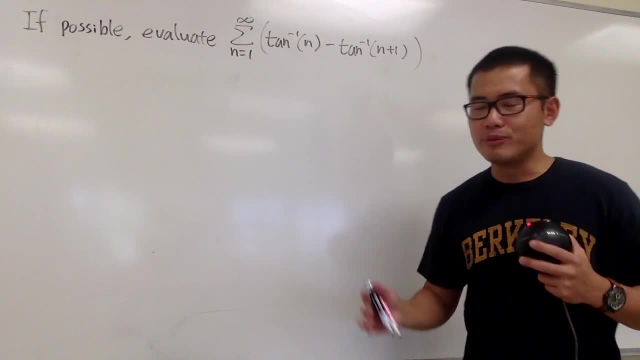 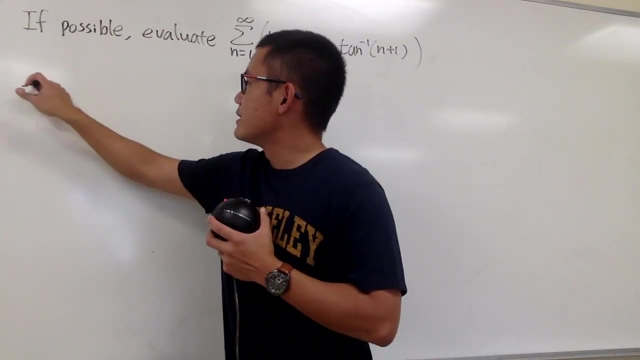 The input here is n. the input here is n plus 1.. So you know this is going to be a telescoping situation, So we will do the usual style. Let's write down a few terms first, alright? So let's see, I'm just going to use this formula here because it's well-written for us already. 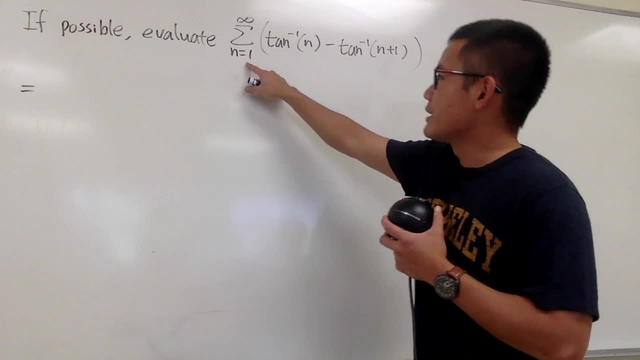 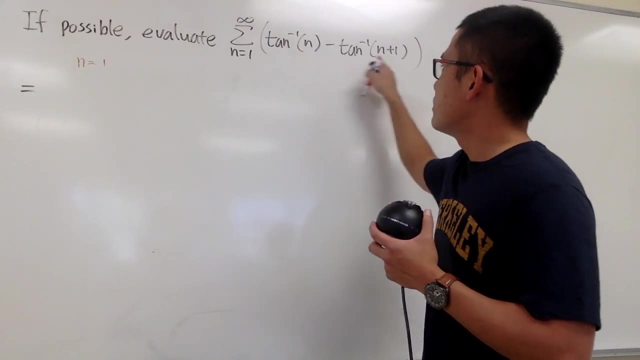 There's not too much algebra we can do, So I'm just going to plug in: n is equal to 1 to here and here, so let me indicate that When n is equal to 1, plug in 1 to here. plug in 1 to here, right. 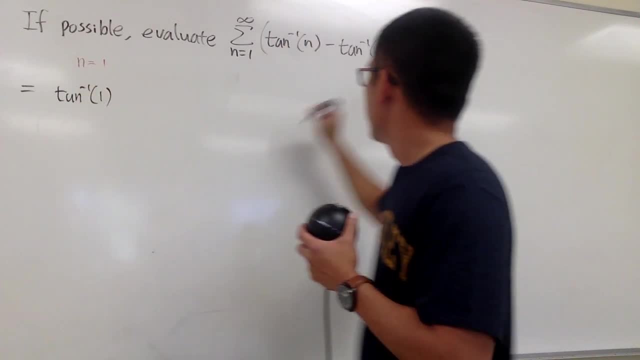 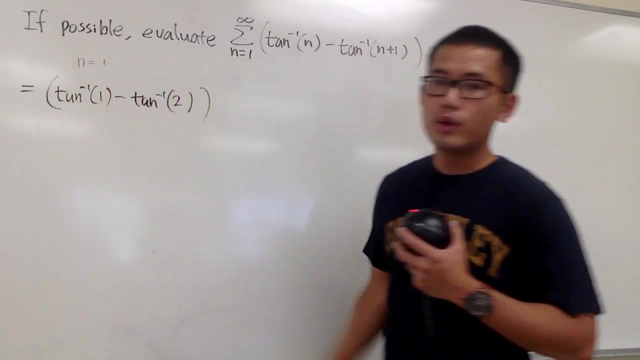 First term we will have the inverse tangent of 1, and then minus the inverse tangent of 1 plus 1, which is 2.. So this is the first term, When n is equal to 1, and then we will be adding this with when n is equal to 2.. 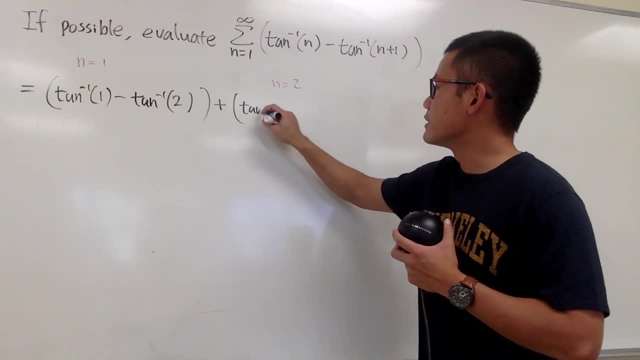 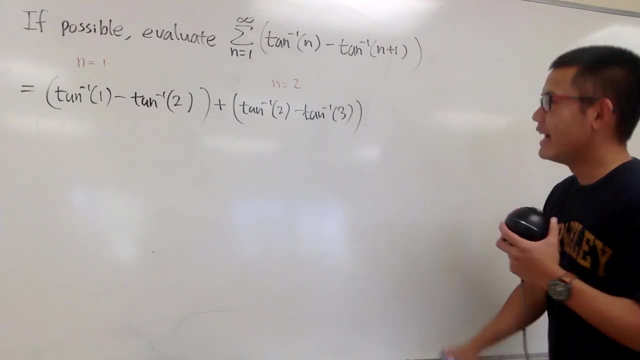 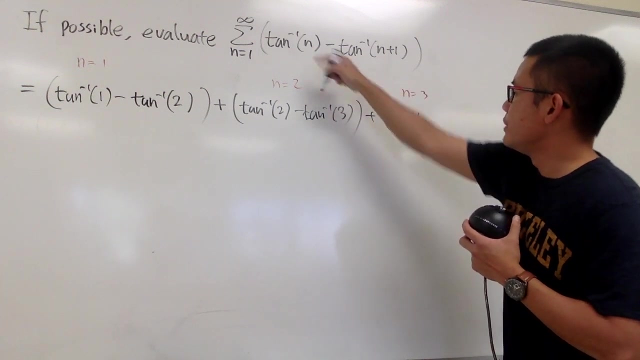 So plug in 2 into here, and here we will have the inverse tangent of 2 minus the inverse tangent of 3, like that right. And let me just put on one more: plus n is equal to 3.. So inverse tangent of 3 minus the inverse tangent of 3 plus 1 is 4, and so on. 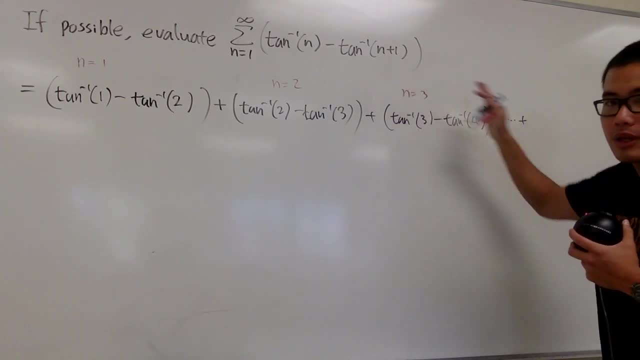 So put on plus, da, da, da, plus. let's put on the formula right here: For the nth term, we will have the inverse tangent of n minus the inverse tangent of n plus 1. And then it keeps on going forever, right? 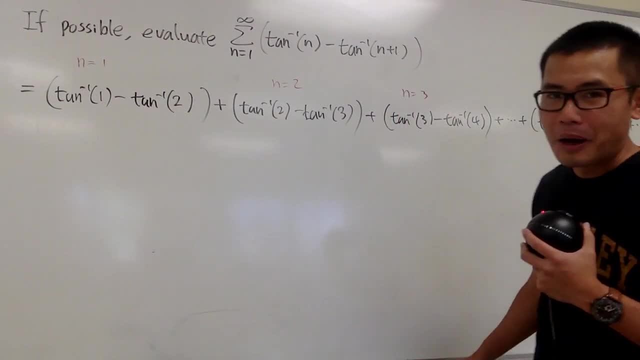 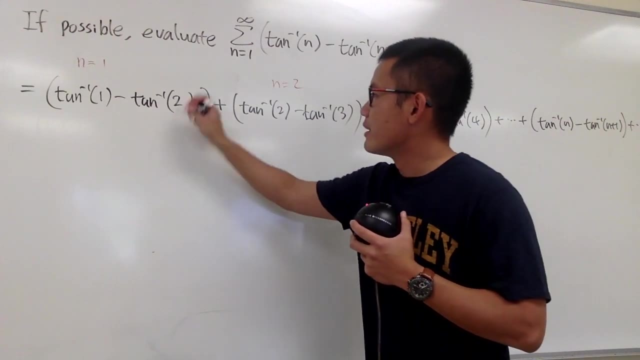 Okay, so I think you guys can all see this. And now here's the best part, the cancellation part. This one stays because there's no other inverse tangent 1. This right here cancels out with this one right away. This right here and that cancel each other out right away. 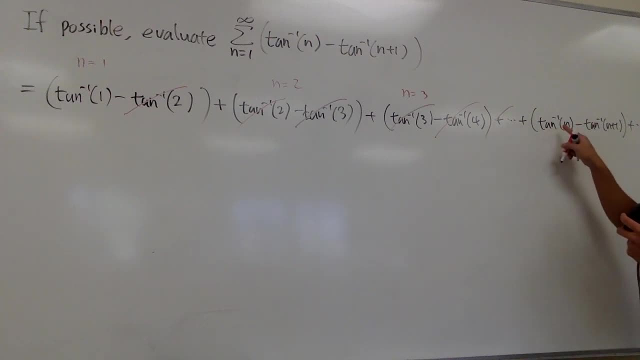 And you know this is going to be cancelled out with that And this is what we have right here, but something in the front is going to cancel out this right. So cancel, cancel. With that being said, we only have that, the actual number, partwise. 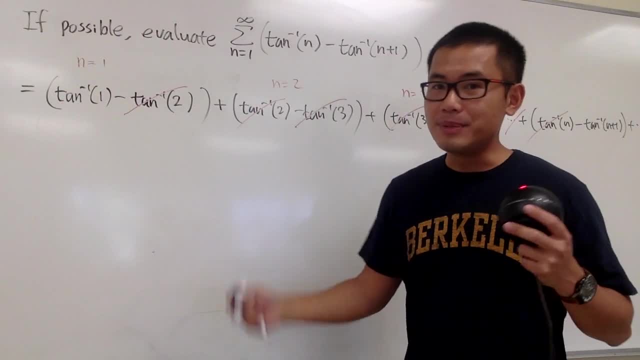 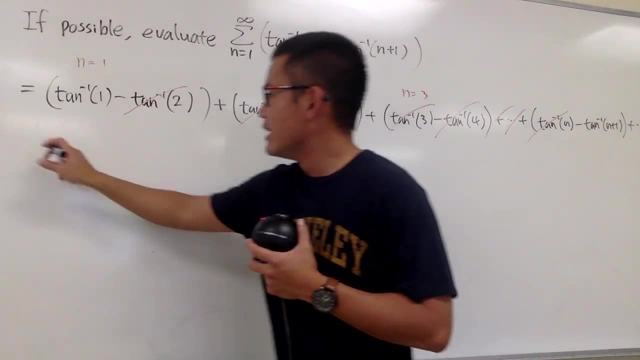 One of this left right. And the reason is because this and that is just off by 1.. So you can expect to have just one term left, the actual numberwise. Therefore, this is going to be The inverse tangent of 1, right. 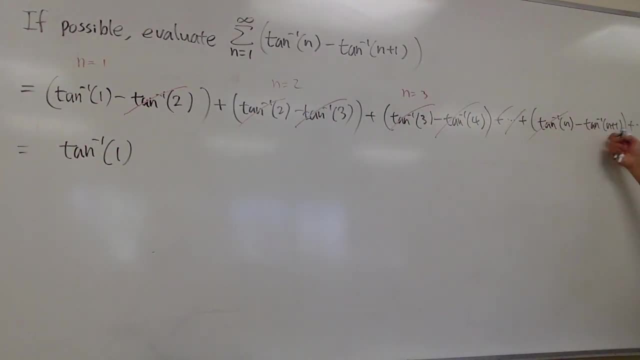 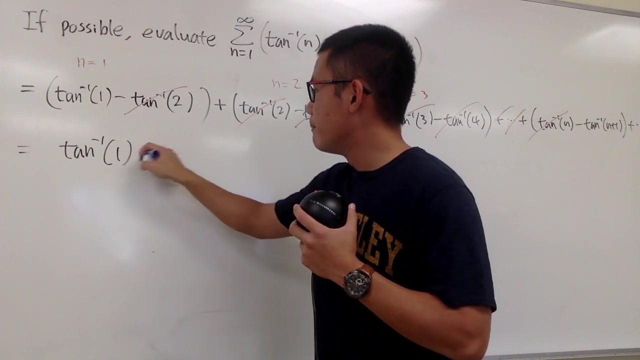 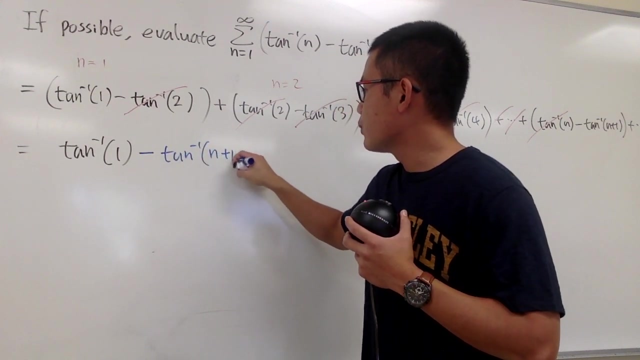 The actual numberwise. However, you must put this down as well. You have to take this into consideration, right? So I will put this down in blue: Minus, right, That's a minus, And we have the inverse tangent of n plus 1, like this: 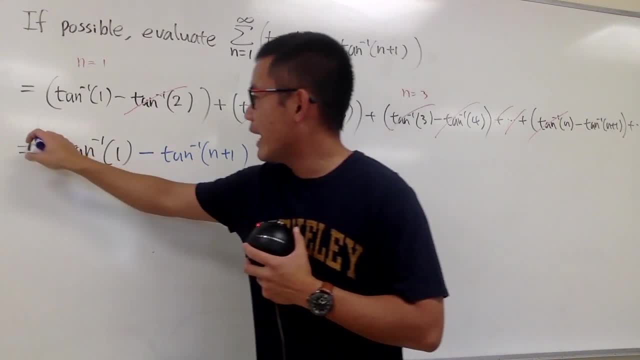 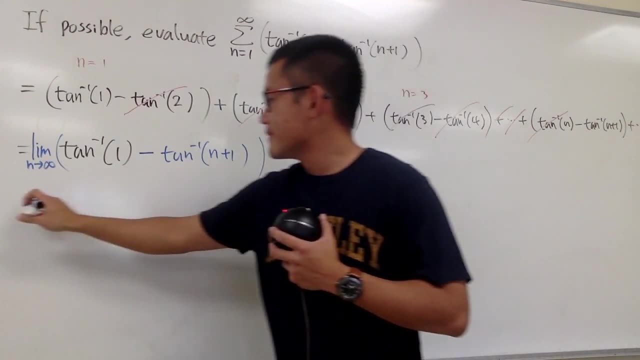 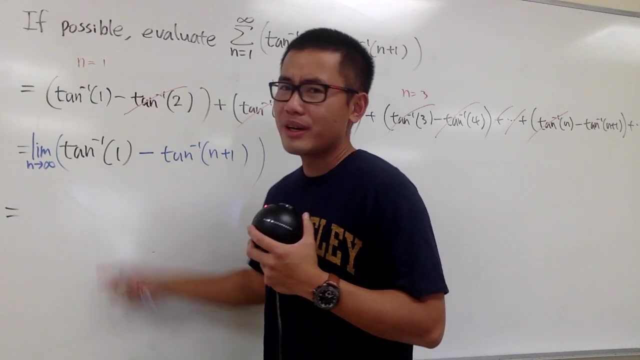 This is the formula part, And we have to see what will happen as n goes to infinity. So we take the limit of this right. Okay, so the first one is just inverse tangent of 1. And we know that we can calculate this right. 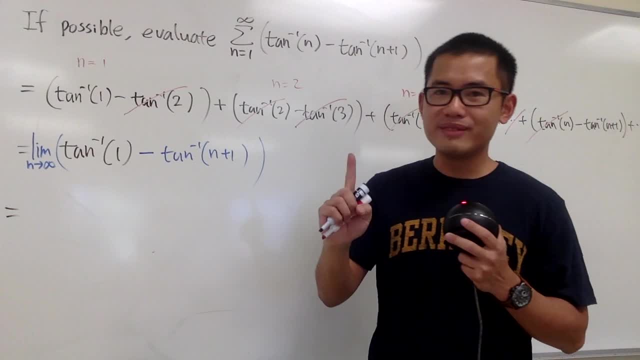 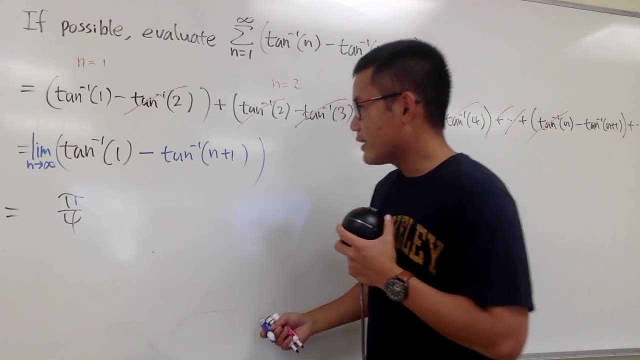 So you have to ask yourself: tangent of what angle will give you 1?? This is just pi over 4, because tangent of pi over 4 gives you 1, right Alright. when n goes to infinity, infinity plus 1 is still infinity. 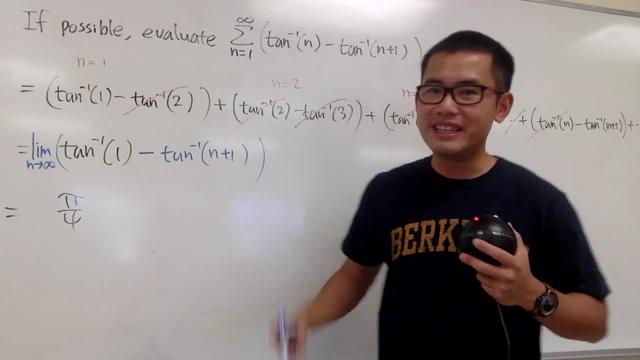 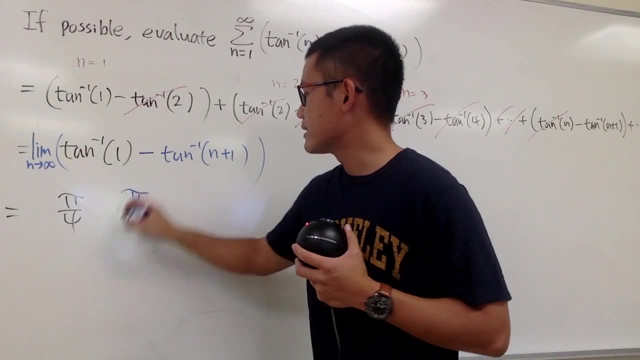 Inverse tangent of infinity is that horizontal angle. That's the limit, that pi over 2.. This right here is going to give us pi over 2, right, And that's a minus. So, as you can see, here we are dealing with finite values. 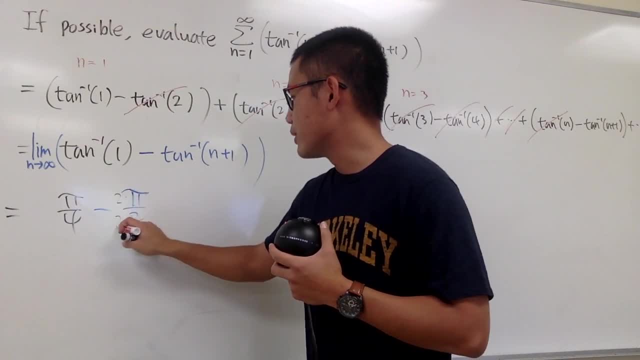 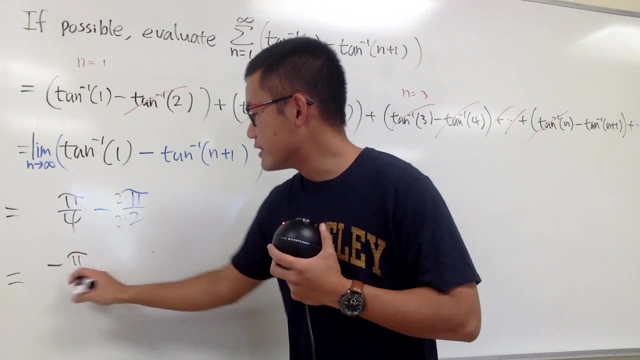 And of course we can just work with this Right here. let's go ahead and multiply 2 and 2. And you will see that this is 1 pi minus 2 pi, So we have negative pi over the same denominator. 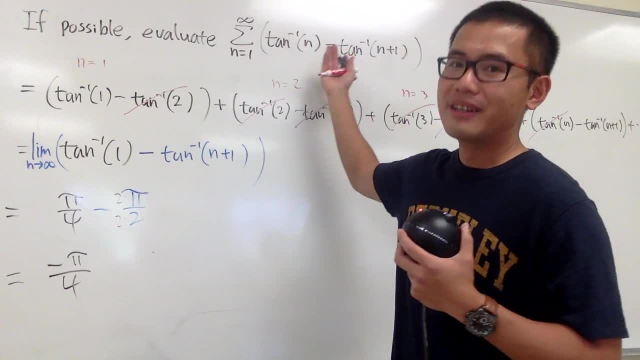 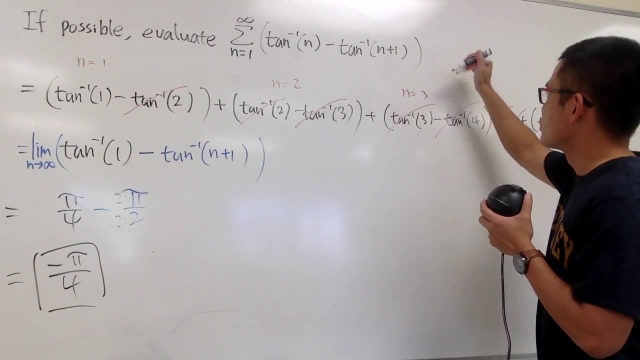 Negative pi over 4, like this. Therefore, this right here converges And it converges to negative pi over 4.. Once again, let me just write this down right here for you guys: This right here It converges. 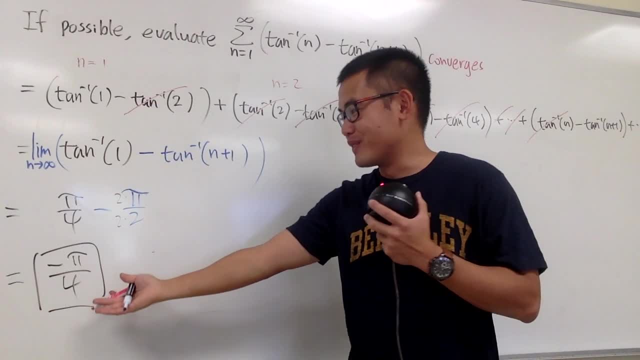 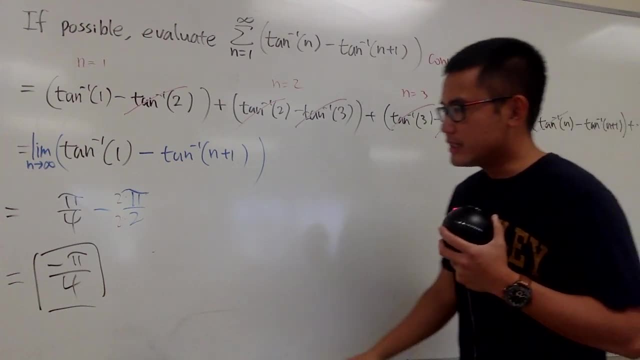 And the reason is because we find the value for the convergence right. This converges to negative pi over 4. It is possible to end up with a negative value because, in fact, this term is bigger than the previous term, right. 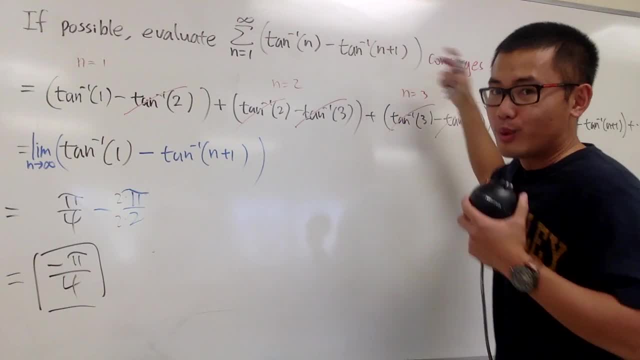 So you just keep adding negative value And it goes along the way infinitely many times. That's the answer. That's it. Telescoping some again. 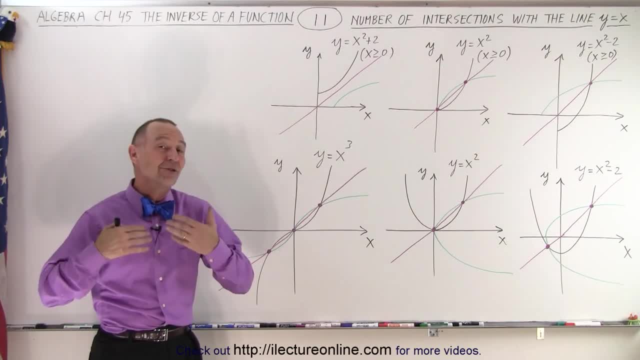 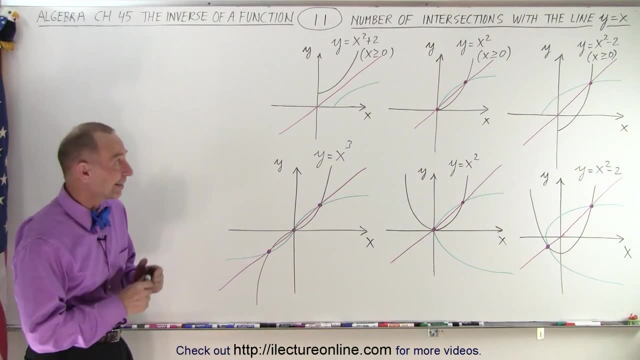 Welcome to ElectronLine To give us a better understanding of what the inverse function is, at least from a graphical perspective, and how it relates to the y equals x line. let's take a look at some of these graphs that we've drawn. Notice that at the top we have y equals x squared plus 2,. 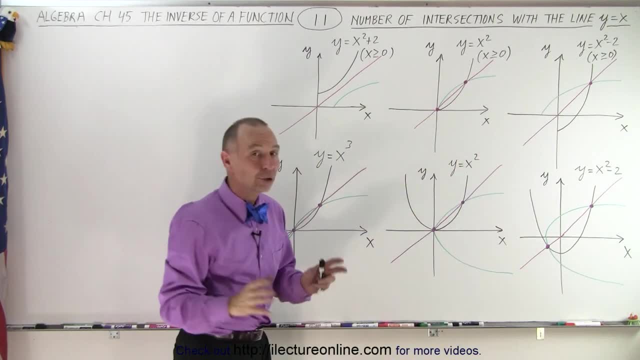 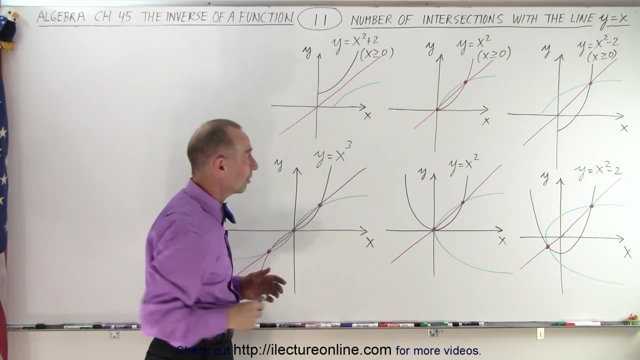 y equals x squared and y equals x squared minus 2, but the condition there is that x must be greater than or equal to 0, which means that we have a one-to-one function in each of the cases at the top. At the bottom, we have y equals x cubed, y equals x squared and y equals x squared. 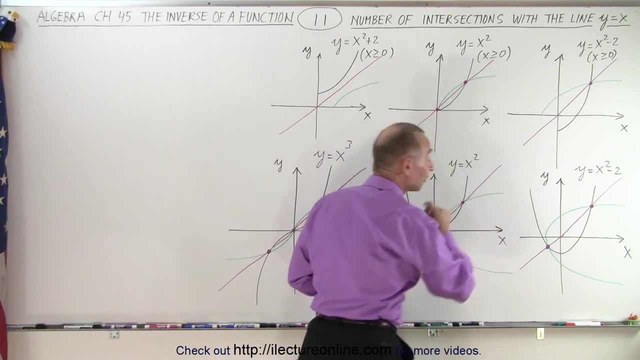 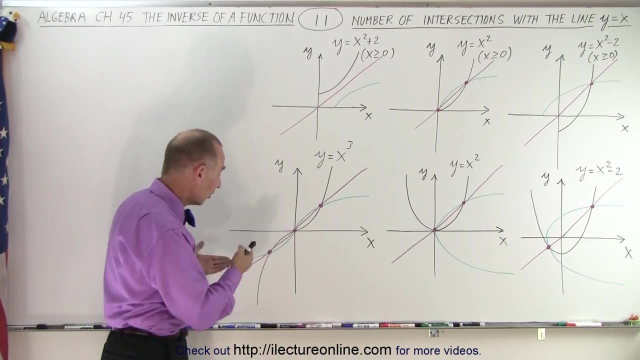 minus 2.. Notice that these two are not one-to-one functions, but this one is: Y equals x cubed. since it's an odd function- x to the third power- it does give us a one-to-one function. We can try the horizontal test and it only crosses the line once. Now notice that if we 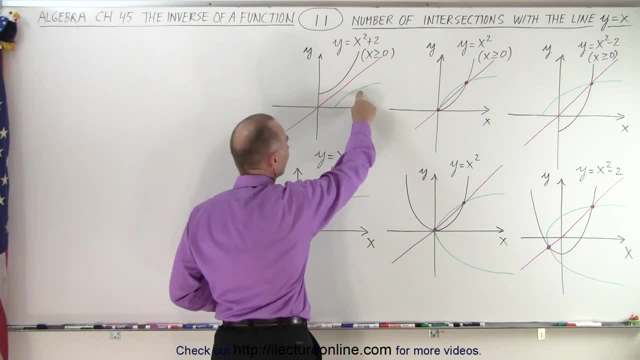 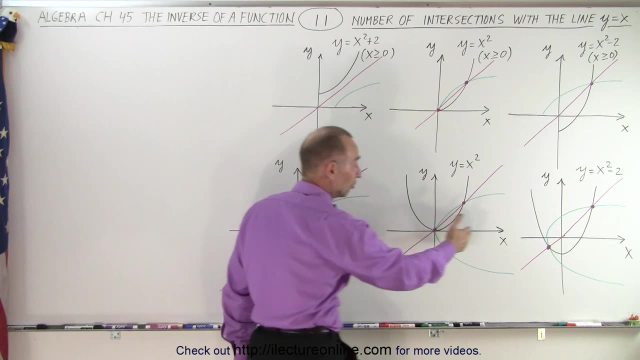 draw the inverse of the function. these are the green lines. there's the inverse of the function, the inverse, the inverse, inverse, inverse and inverse. Notice that in these two cases, right here, the inverse of the function is not a function, it's a relation. because we did not. 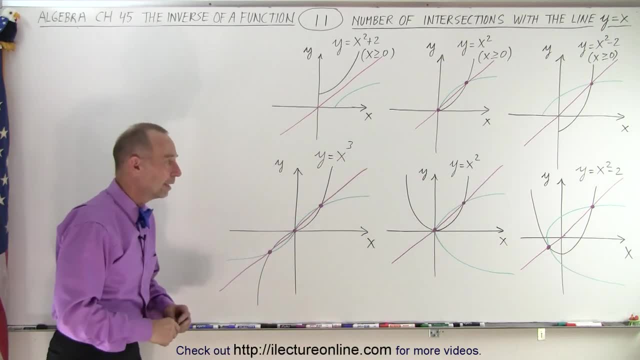 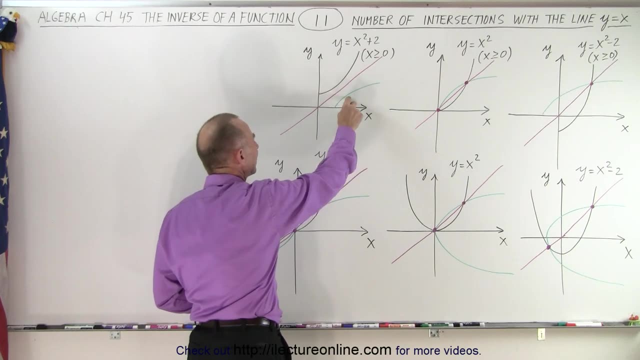 have a one-to-one correspondence or one-to-one function of those two examples, But we're interested in where the function and the inverse of the function cross the y equals x line. Now here you can see that it does not cross the y equals x line, not even once Here.